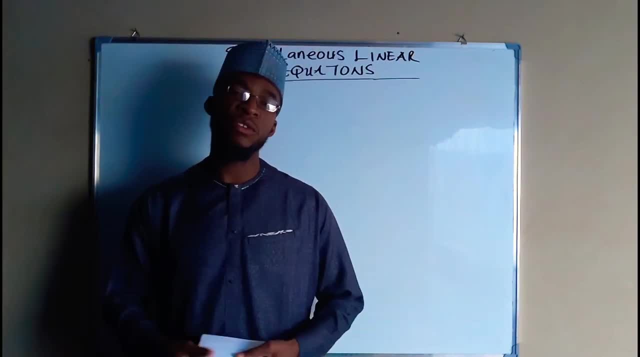 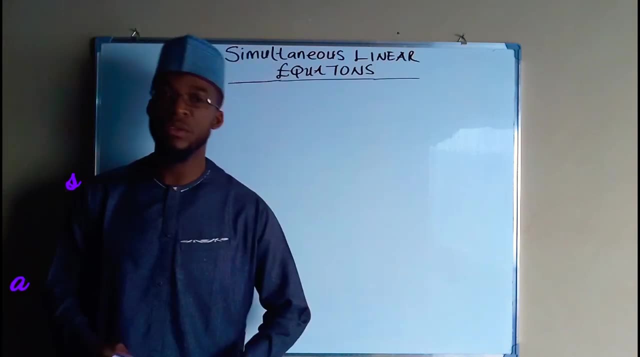 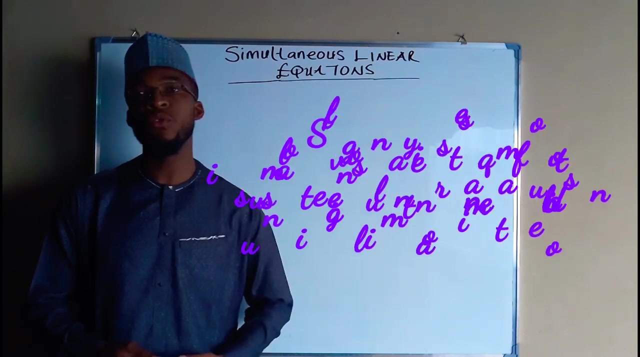 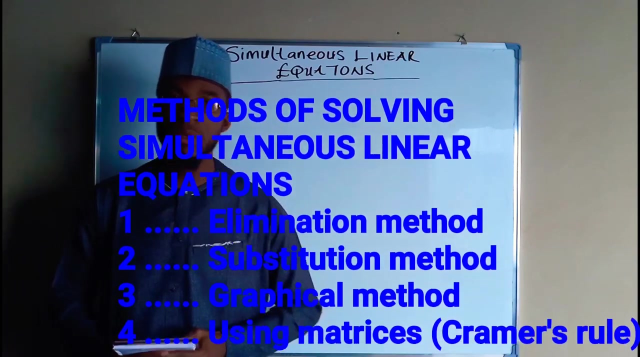 hello, good afternoon viewers. welcome to another edition of my tutorial. in this chapter we are going to be talking about simultaneous linear equations. in this chapter, again, we are going to consider the four major methods used to solve simultaneous linear equation, which are the elimination method, the substitution method, the graphical method and, lastly, using matrices. but in this video we are 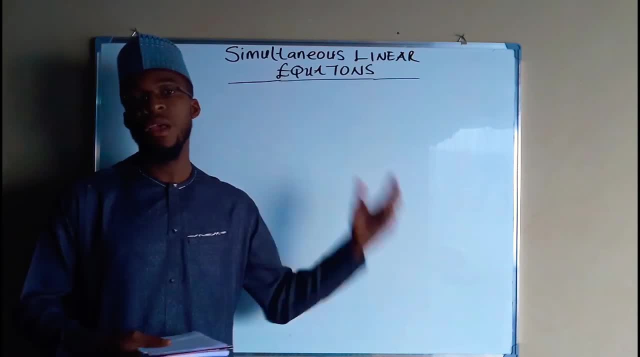 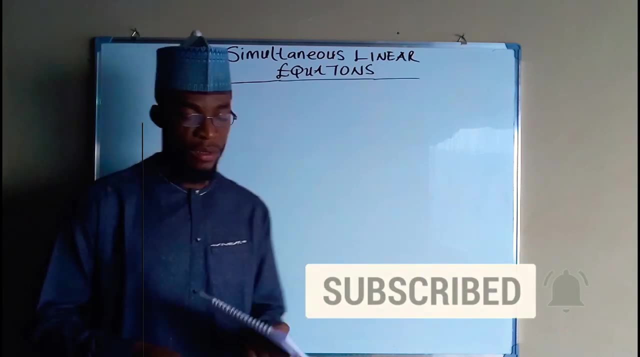 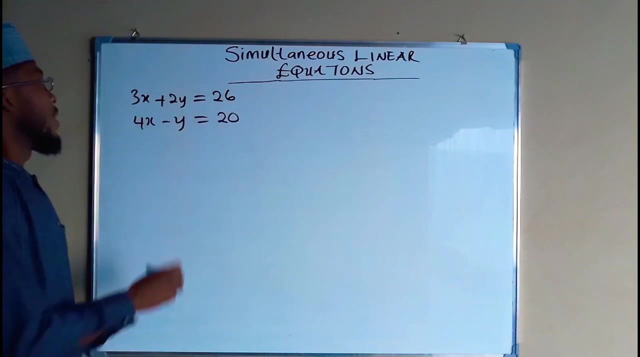 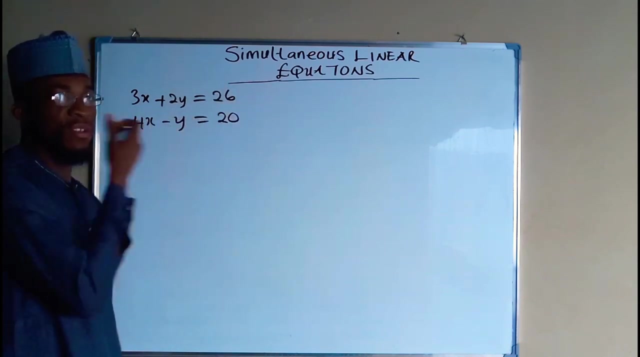 only going to center our discussion on the elimination method. if you are new here, kindly subscribe to our channel. press the bell icon so that you won't miss anything. so first we are given, we are going to find the value of X on Y which will satisfy each of these equations. begin solution: let us call this equation number one, and. 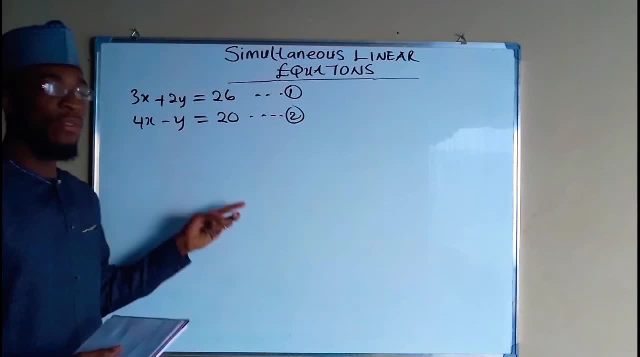 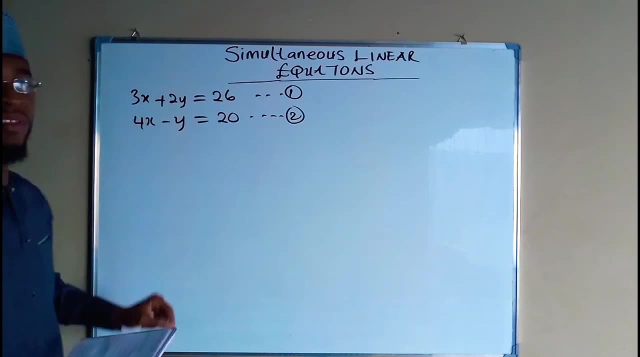 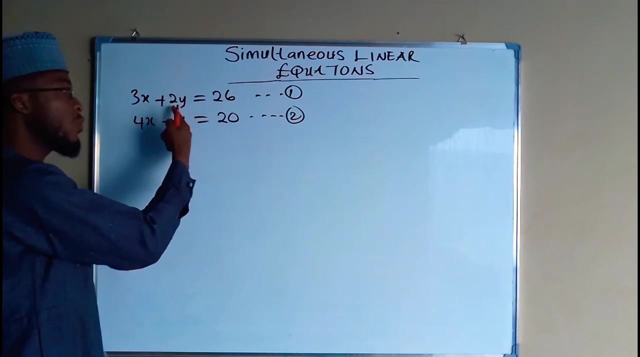 call this equation number two. in elimination method, you are expected to make the coefficient of one of this variable the same. you either make the coefficient of X in equation one and equation two to be the same, or you make the coefficient of Y in equation one and equation two to be the same. so for this, 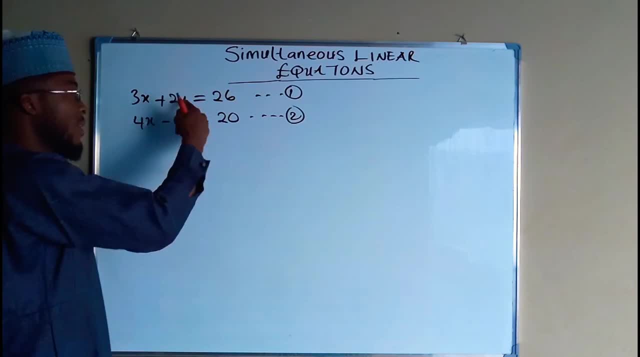 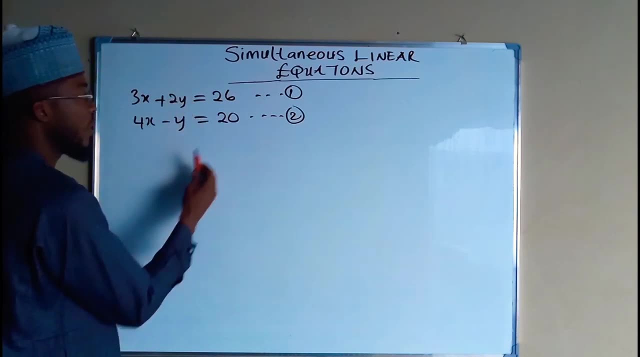 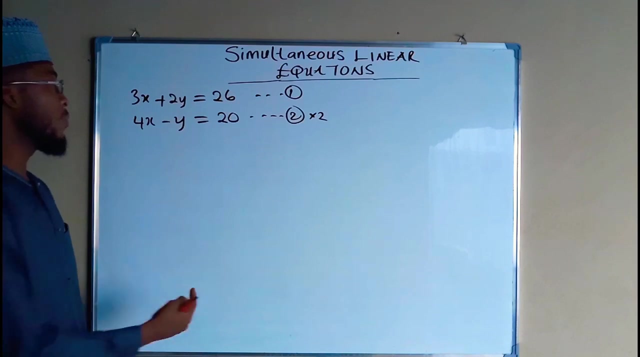 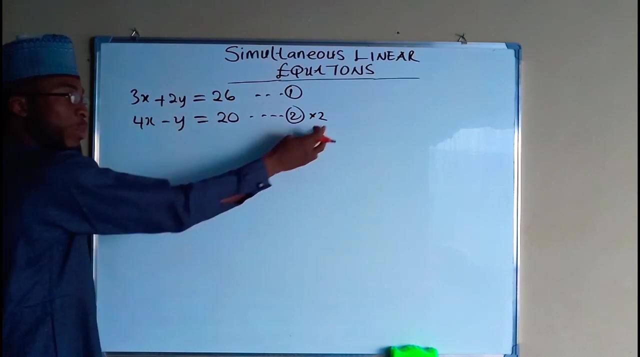 we are going to eliminate Y by making equation one and equation two, both having the coefficient Y the same. if I multiply equation two by two, definitely I am going to have two Y in equation two, which correspond to two Y in equation one. so each time is going to be multiplied by two. the first time here is four times two is going to give. 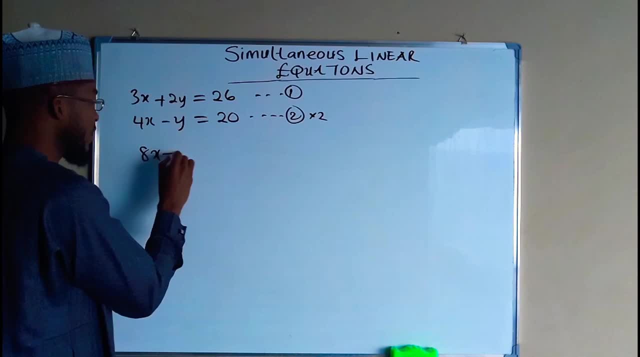 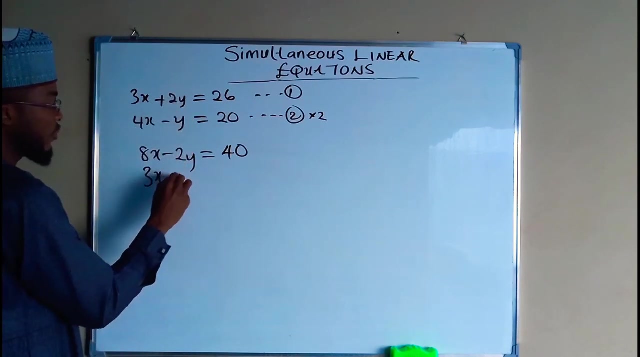 us. the second time is negative Y times two is going to give us negative two Y, and this is equal to 20 times two, which is equal to 40. now we bring equation one back without changing any value there, because what we are after is to have the same coefficient of one. so here we have 3x plus two. 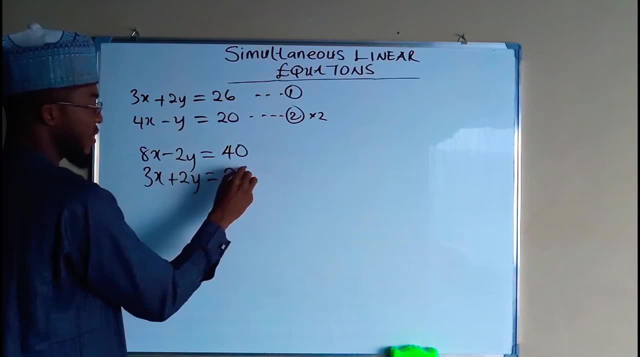 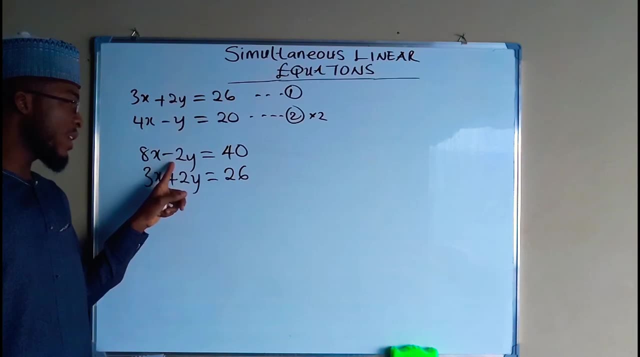 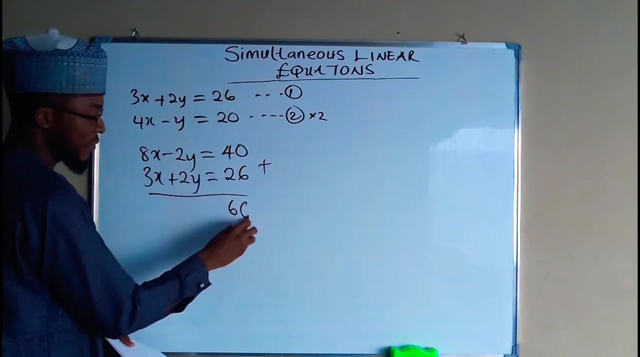 Y, this is equals to 26.. now we want to eliminate Y. so because two Y here is negative while the other two Y here is positive, so if you add them together you are going to get zero. so we add equation one, equation one by equation two. so this plus this is going to give us 66.. 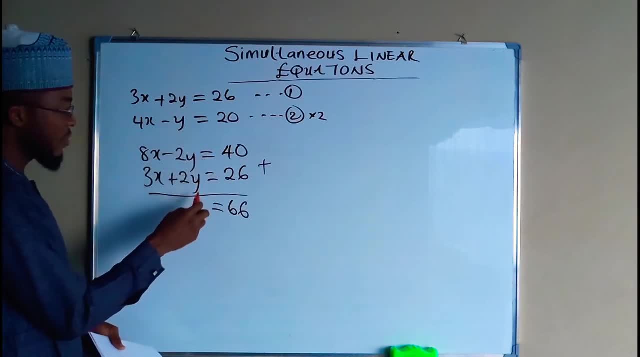 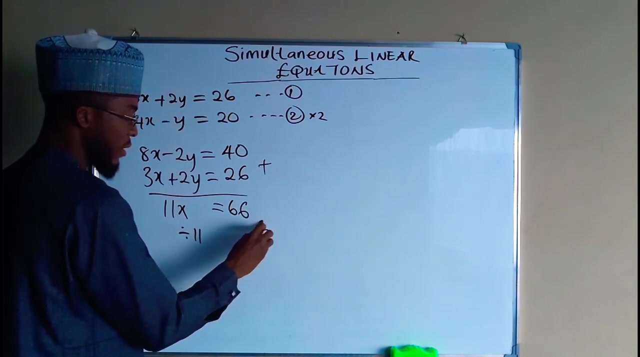 this is equal to: if you add this one together, you are going to get zero. then you add 8x plus 3x and this will give us 11x. now we need to divide each side by 11. divide each side by 11 so that we have. 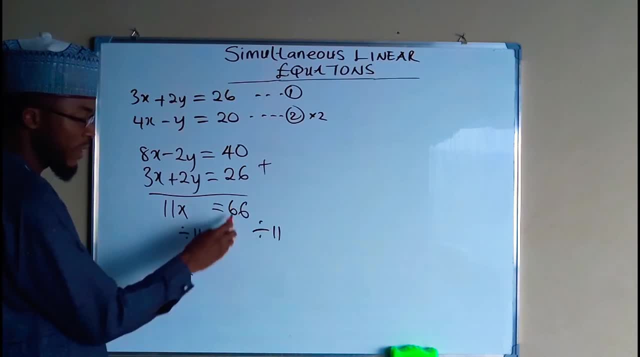 the value of X. so now X is equal to 66 divided by 11, which will give you a six. now we have found the value of X to be equal to six. now we need to find the value of Y by substituting the value of X in either equation one or equation two. in equation one we have 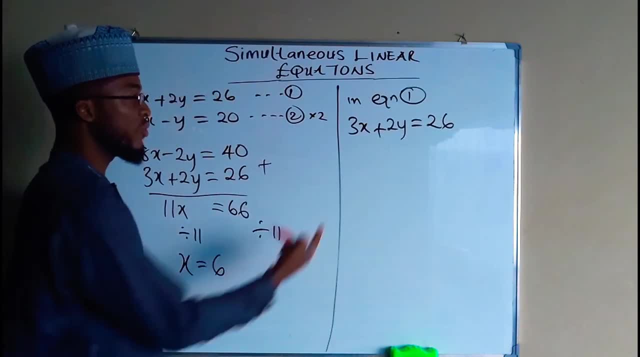 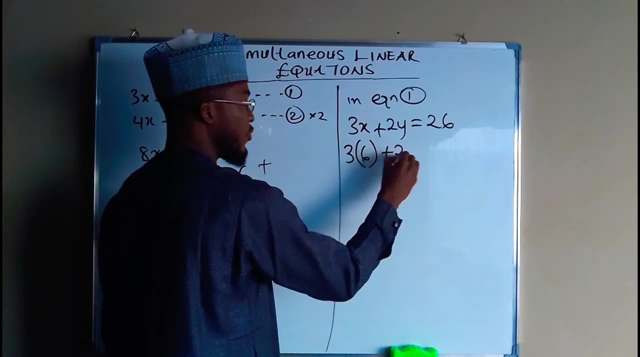 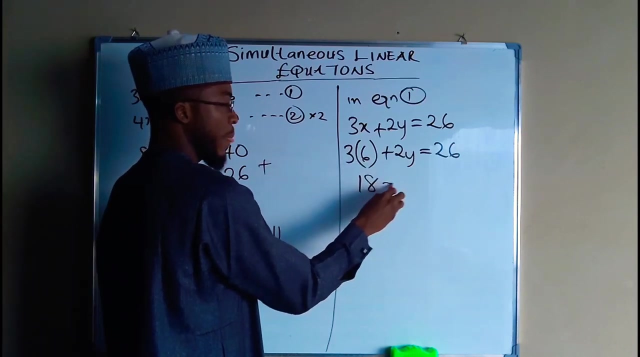 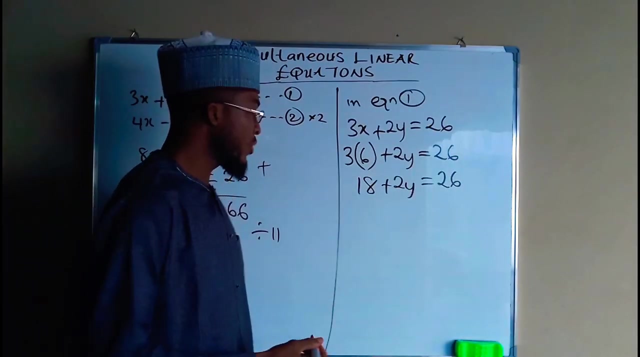 but the value of X is now equal to six. so we substitute the value of X to be equal to six. so we have three multiplied by six plus two Y, and this is equal to 26.. this time this is 18 plus two Y. this is equal to 26.. now subtract 18 from both sides. minus 18, minus 18. 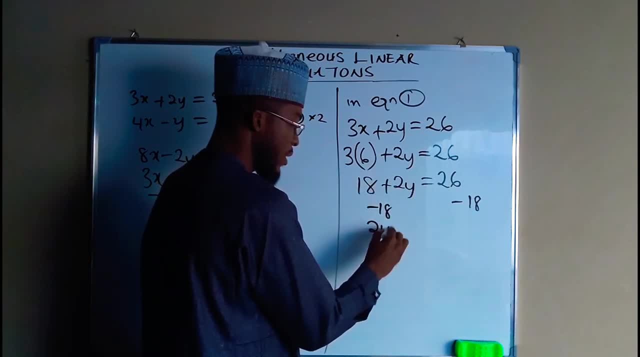 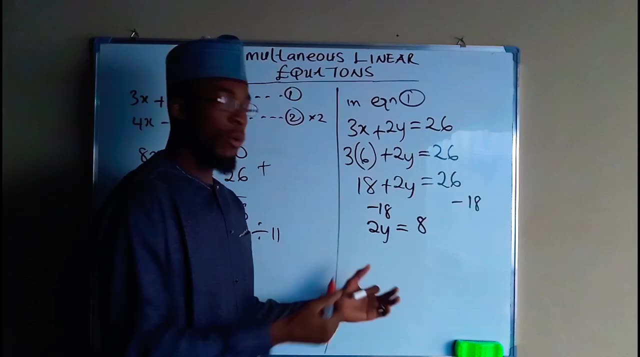 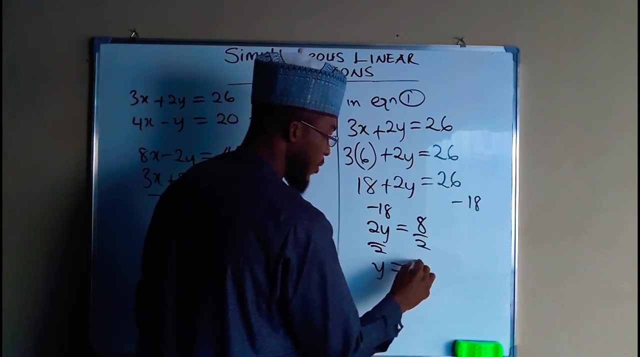 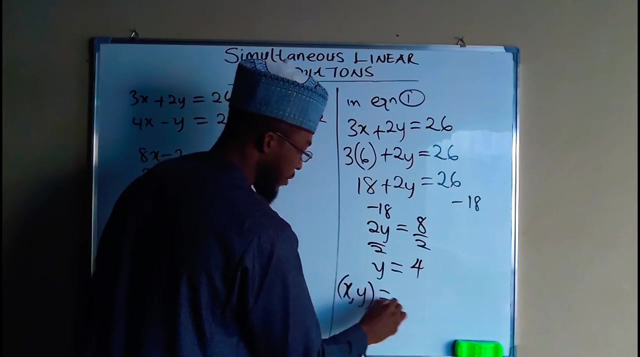 uh, 18 minus 18, zero. so we have two Y on the left hand side and 26 minus 18 is equal to eight. if you divide both sides by two, by two, you end up having the value of Y to be equals to four. so now the values of X and Y are: X is equal to six, Y. Y is equal to four.